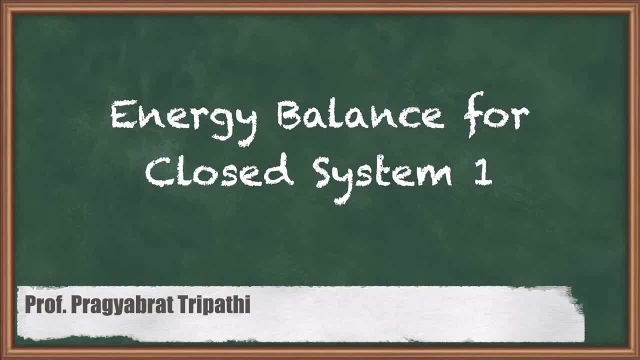 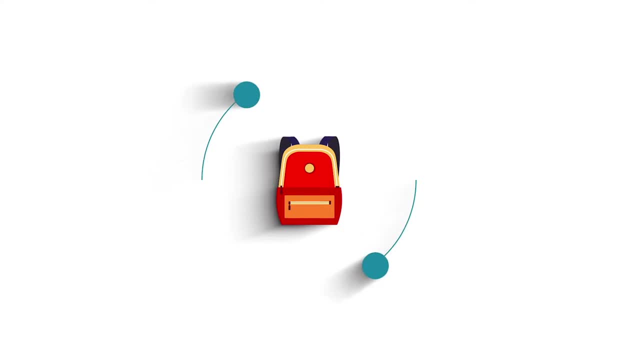 Hello, my dear friends, in this video we will going to learn about energy balance for a specified system that is a closed system. so, as we know that the system is closed, that means fixed mass of the system, fixed mass of the system. right, fixed mass of the system. that means there is no any flow of the mass flow. 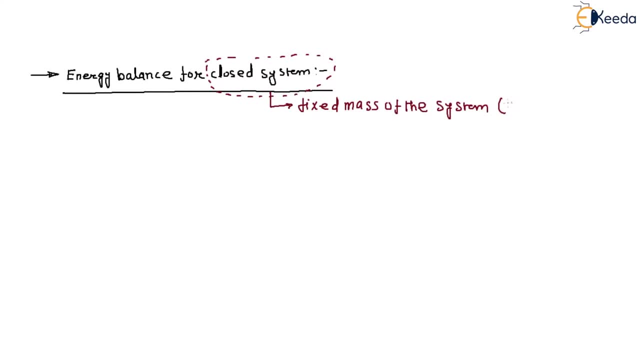 across the system. boundary that means there is no any change in mass is zero, right. so if there is a system, if there is a system that means there is no any flow of mass, right, that means only flow either heat and water, right. so this is a closed system now. so in. 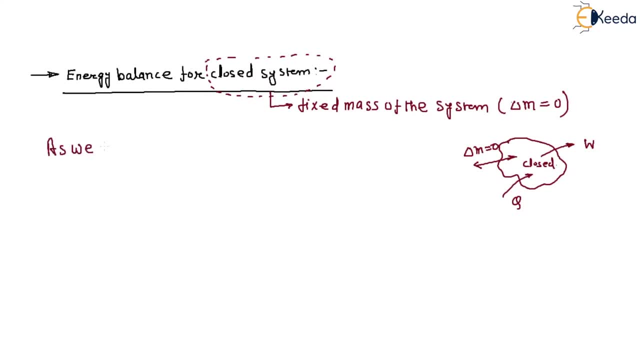 general, as we know that, as we know that the energy- that means energy in minus energy out, that means energy transfer- is equal to change in total energy of a system. this energy transfer is due to heat work and mass and this energy change of the system is either I is internal energy, kinetic. 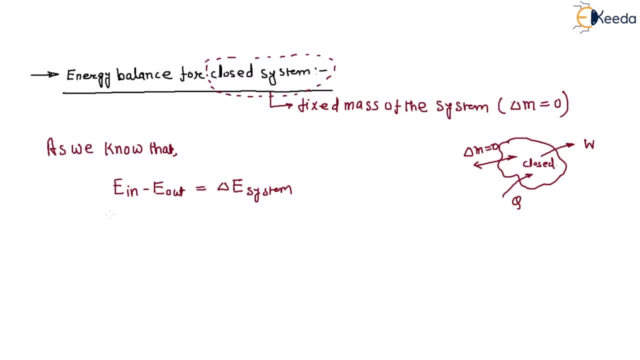 energy and potential energy. so this is for any system, for any system and any process in general. this in general. but if the energy is in the form of heat, energy, out in the form of work, and this system, energy is equal to Delta U. so this equation, this equation, this equation is applicable, this equation is applicable. 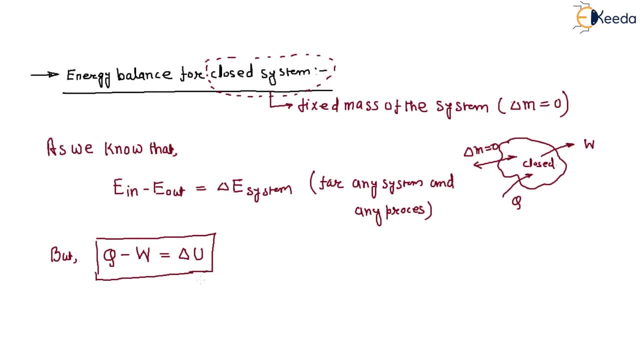 for what? what is the assumption of this system? tell me what is the assumption. this is your number first, very important. I am telling you number first, first law for any process is your first law for any process, right number second: what is the second assumption for closed system? closed. 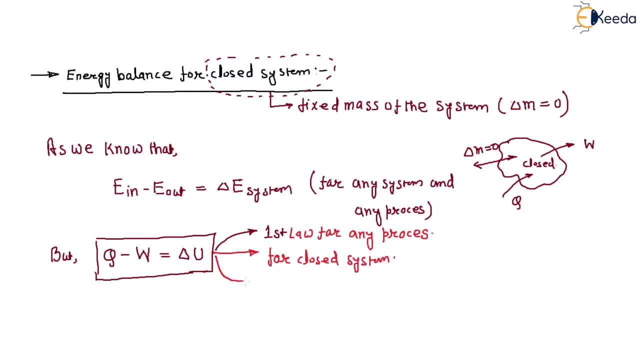 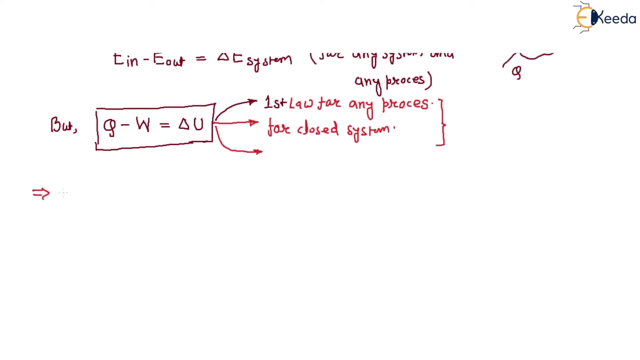 system, or also called stationary and number. third right: this is the sufficient. this is the sufficient right. this is your first law for any process and for closed system. right DQ, so you can write for a process, for a process 1 to 2. how can you write this equation? Q 1 to 2 minus W 1 to 2 is equal to U 2 minus U 1. 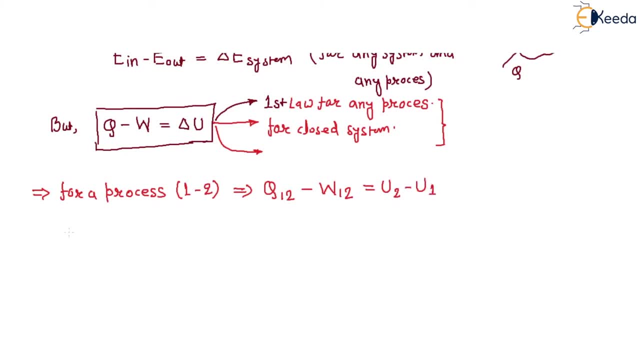 this is for process right in the differential form. that means you may write also in the form of differential form. differential form: what is that? DQ minus DW is equal to delta. this is in the form of differential form. right now you can also write: Q minus W is equal to delta. these all are the different form. 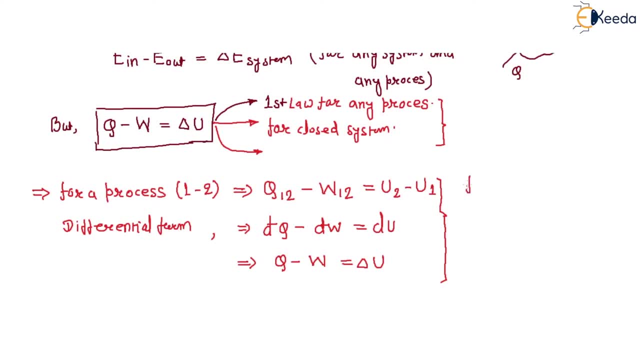 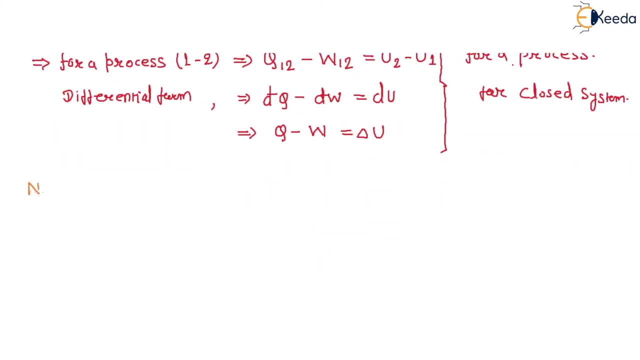 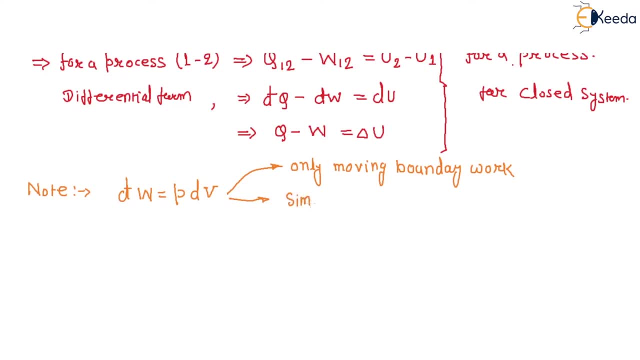 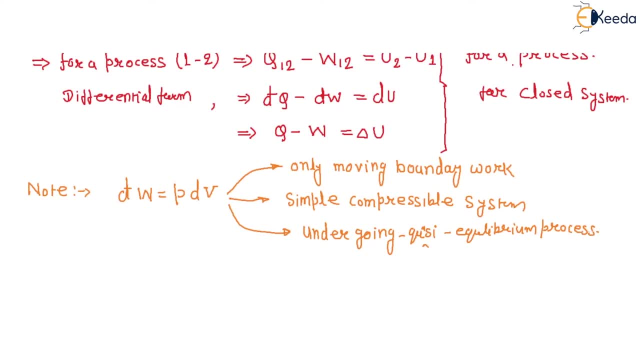 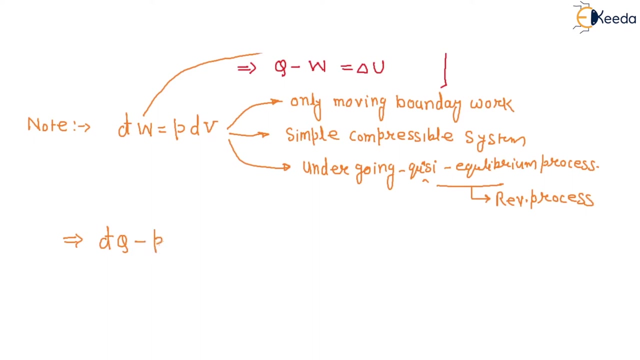 process- that means quasi-equilibrium process- is generally reversible process. so if you put this dw here, if you put this dw here, so the equation- it is in the form of dq-pdv- is equal to du right. so this dq is equal to bu plus pdv. so what is the assumption? 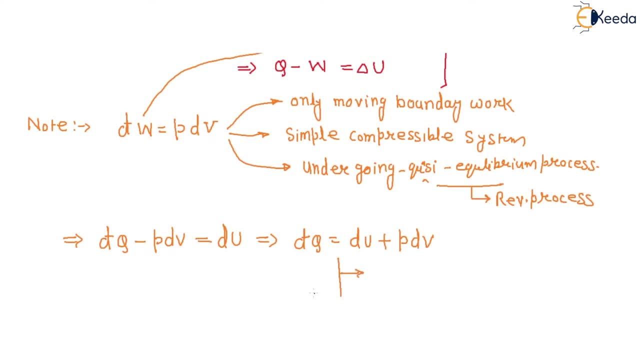 here. The assumption here is that this is the first answer of the equation. So this is the first one. first law for closed system. why? because there is a DU, now other neglect. the change in that means stationary system, closed system. that means, in this neglect, change in kinetic energy. 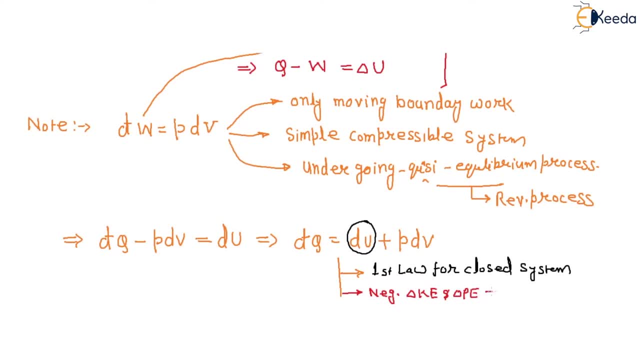 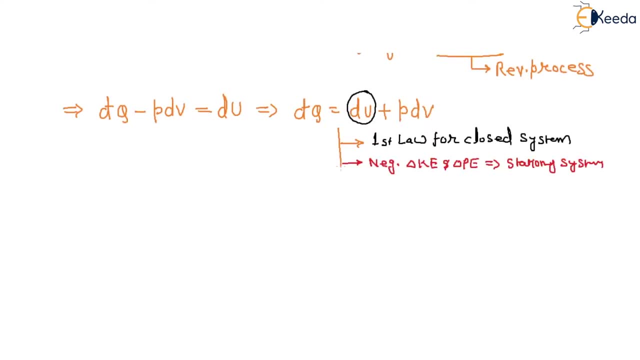 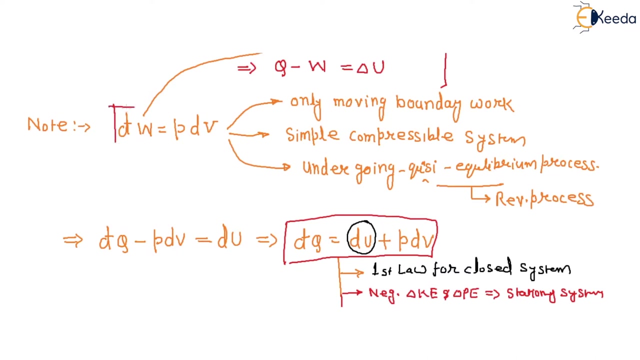 and change in potential energy. that means a stationary system. other is that. what other is that? a reversible process? one way, not any process. that means quasi static, ecclesiastical equilibrium, right? so keep in mind what is the validity of this equation and what is the validity of this equation? this is. these are very important. I am telling you many books. 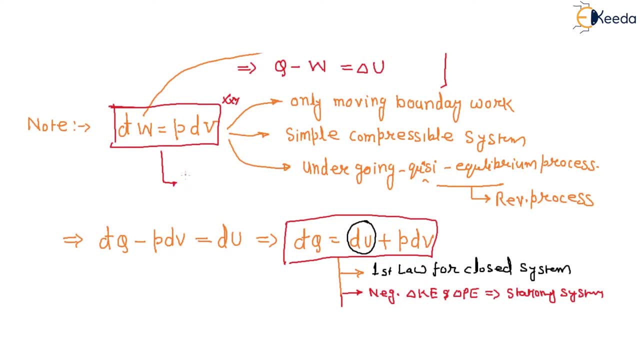 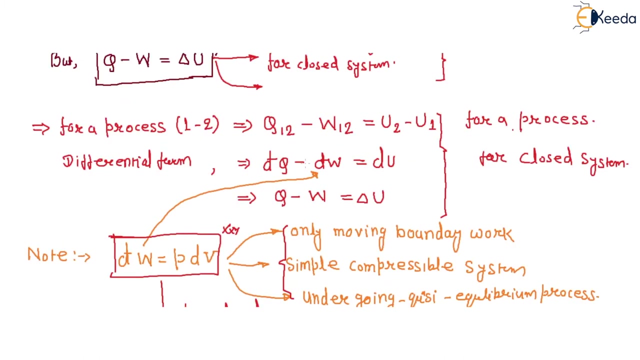 this gives for closed system, for closed system, which is wrong. this is for any system. only assumption: is this only assumption? this, that means only moving boundary work, simple, compressible system undergoing a quasi equilibrium process. that's it, which is not need to say that this is open system, closed system, no right, ok, ok, so DU, and for this? 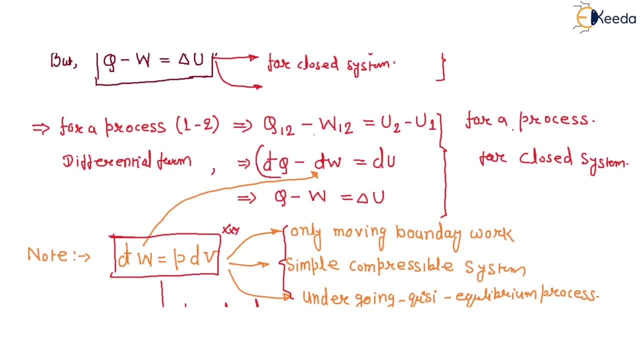 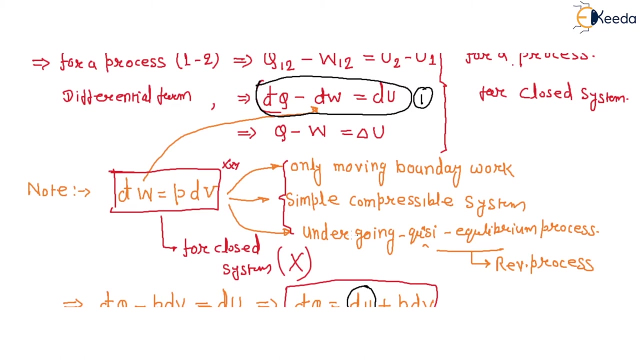 this is also important. this three equation are important. this three equation are important. number first: what is the assumption of this equation for any process closed system? right, for any process closed system. what is the assumption of this moving boundary work, simple, compressible system undergoing a quasi equilibrium process right. number second: number three: this is also important. 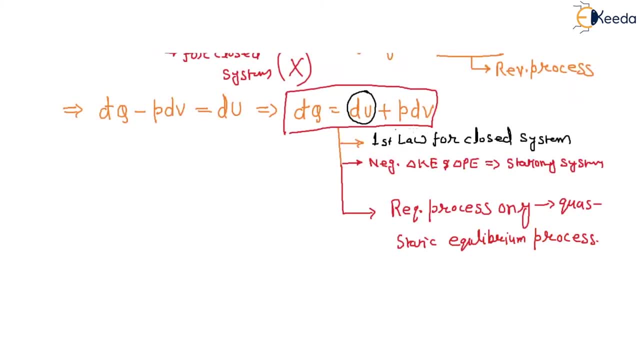 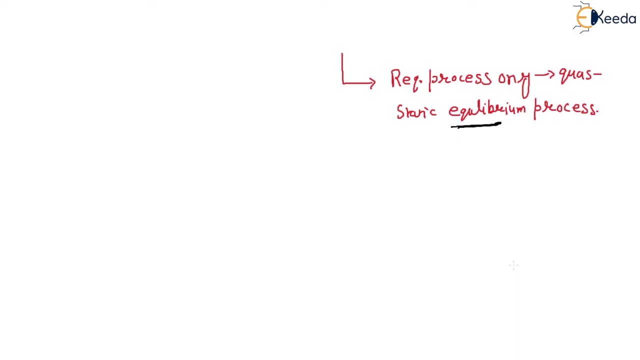 number third: what is this first law for a closed system? stationary system, neglect, change in kinetic and potential energy, and this is your quasi equilibrium process. that means a reversible process. ok, so this is your first law for a closed system or process. now, if you take a example like: 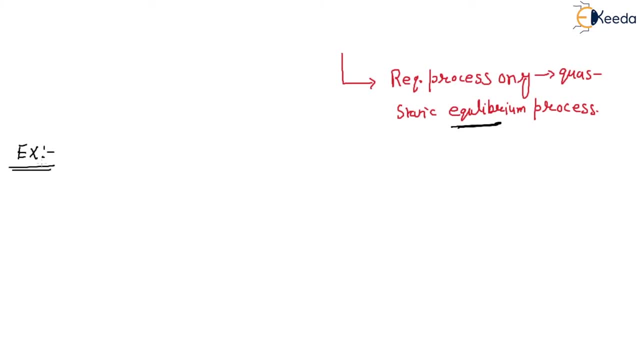 that, see, see, a well insulated, rigid tank. there is a tank, well insulated, a rigid tank. so there is a tank. so this is your tank, are insulated, mind it, this is your insulation tank, right? so this is your insulation tank. so, what is given? what is given, rigid tank. 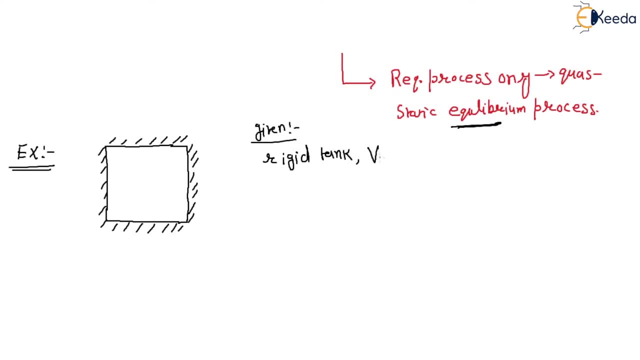 what will be the impact here? because if it is insulated we have a fixed tank. will we put diatomite OR so unchanged volume of the tank is fixed. that was change in volume is equal to 0. rigid tank. okay, number fast. the volume is 1 meter cube. this tank have a volume 1 meter cube right contain 1 kg. 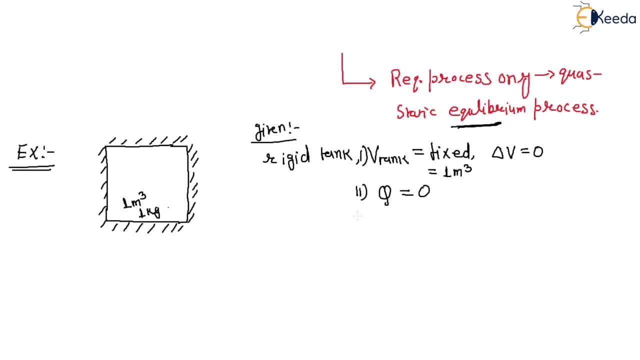 of an ideal gas. that means mass of gas is given 1 kg ideal gas. ideal gas have a constant cp and cv volume of p approximately. so cp is given 1000 joule per kg kelvin and cv is also given 800 joule per kg. this is given number third. now at a pressure. what is the pressure here? 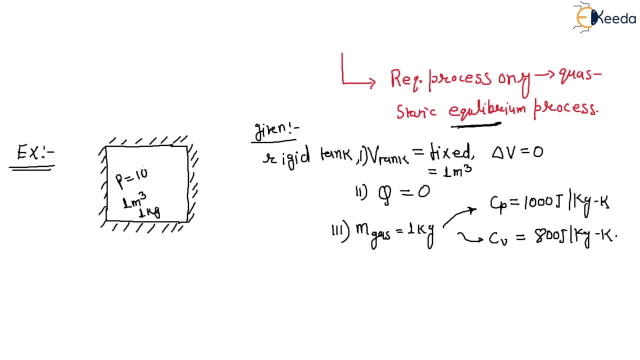 the pressure is 10 to the power, 5 parts the pressure. this pressure gas. a stirrer is rotated at a constant rpm. so there is a stirring device. so there is a stirring device if your stirrer is rotated at constant rpm. fixed rpm is fixed rpm. say so if a stirrer is rotated. so in this system, 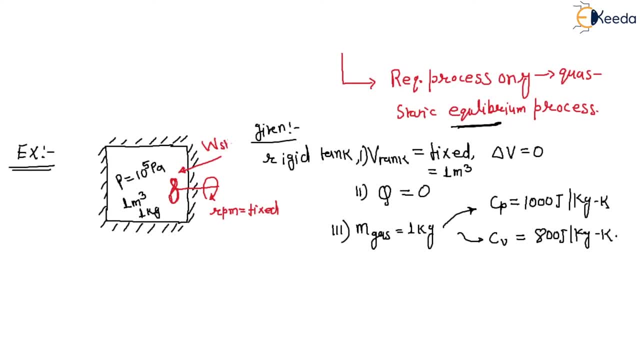 we have work supply, which work soft, work right. and what is the rotation? this rotation is thousand rotation. constant rpm of a container has a thousand rotation, thousand rotation, thousand, one thousand, process and apply a torque. and what is the torque is given torque is applied: hundred newton meter. this torque is applied by the motor. the final. 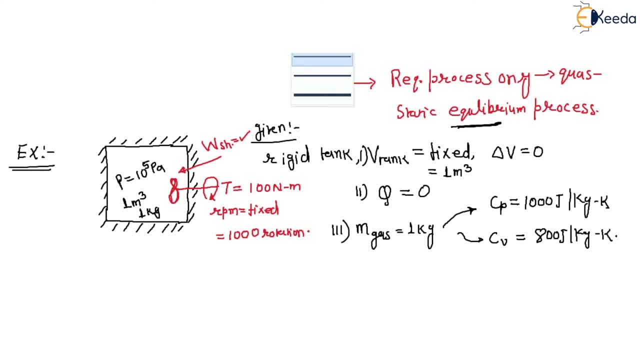 temperature of the gas. so, my dear student, this: before the stirrer of the system, lets its property is 1 and if a star of the system, the property is changed, let, true, why this property is change, why this property is change, why this property is changed. so why, very important, why process 1 to 2? because of that means there is 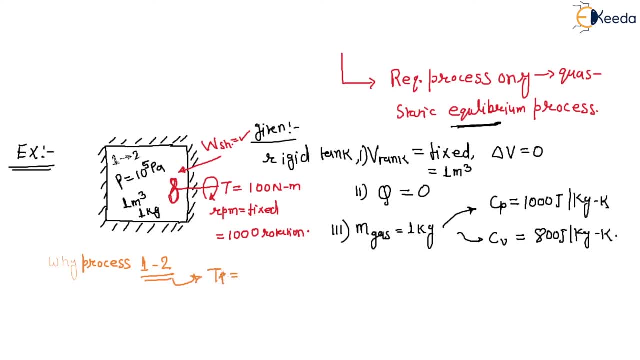 an initial temperature Ti is someone T1 and its final temperature T2. so why this temperature is changed? because of fluid friction. fluid friction: so if you rotate the stirrers device, so the gas energy will increase and that energy will convert it into intramolecular energies. why? because there 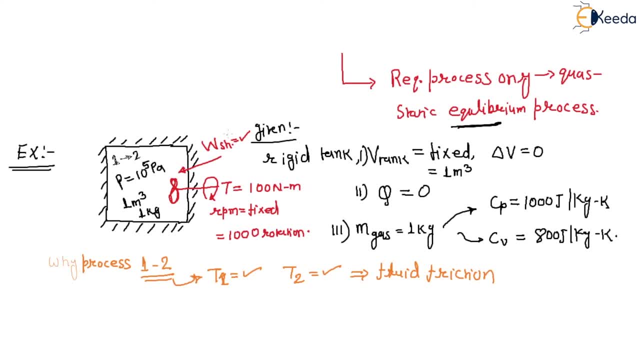 is no any chance why? because if we put a work, so if we see we know that Q is equal to Q minus W is equal to Delta u and delta u is equal to delta u and delta u is equal to delta u and delta u is. so there is no any heat supply and this work is negative. so minus of minus W sat work done on the. 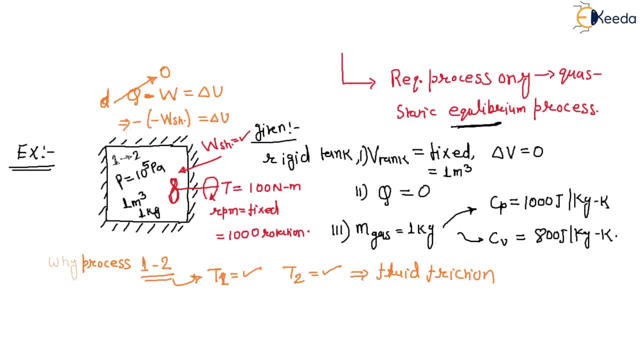 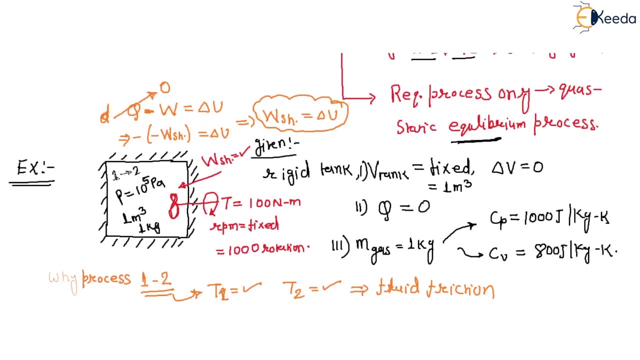 system is equal to Delta u. so if we supply a work with a stirrer system, all work going to the change is internal energy. so this work is added to the internal energy, so this work is added to the system. this is our system, mind it. this is our system. this is our system, this is our system, right. 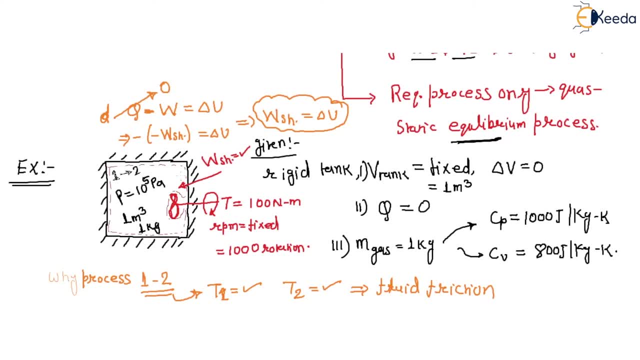 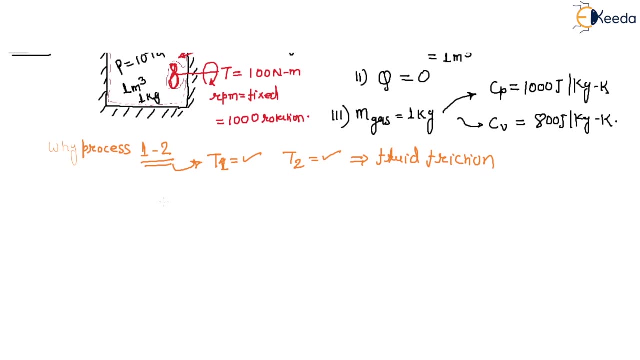 this is our system, so you are giving the energy to the system, the system giving energy, so system gain energy. if the system is gain energy, so its internal energy will increase. so if the internal energy will increase. and we know that for ideal gas, for ideal gas, internal energy is the function of temperature, so its temperature increase. so what? 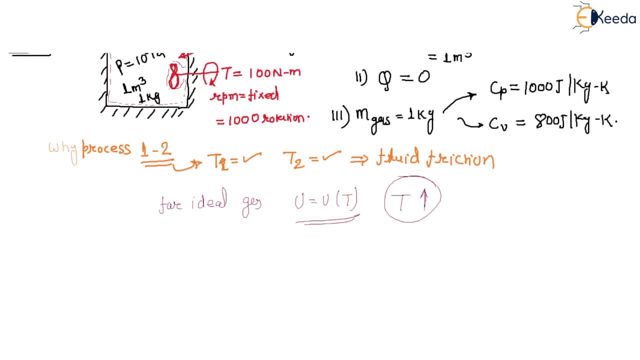 is its increase, the temperature, the question asking like that, right in Kelvin. so first of all we find what is the initial temperature. so delta T is nothing. this is T 2 minus T 1. so well, the only speed that T 1 give this T 1 is I is given and is given that M1 is given. 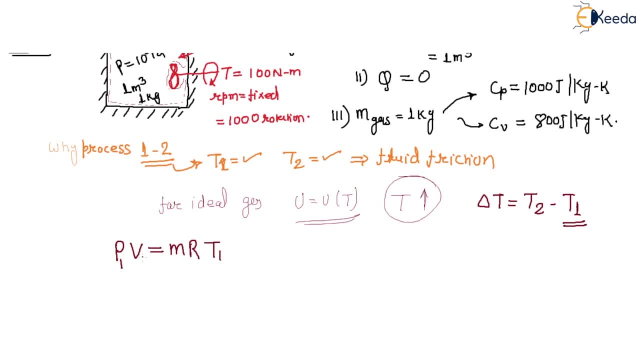 so what is the T 1 see? initial pressure is given, volume is given, M is given, R is given and T 1 initial pressure volume is same RT scal. so for a closed system, closed system- there is no any change in mass. so M1 equal, M2 equal to M, then weapon is T. 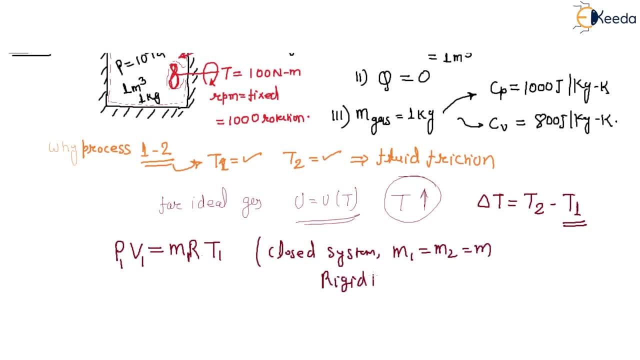 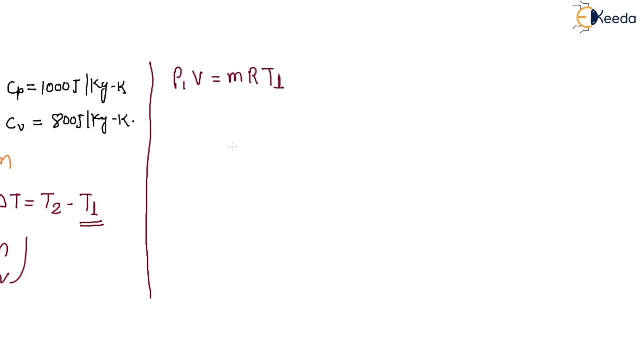 Reset time. So V1 is equal to V2 is equal to V. So what is the equation? So we can write like that: P1, V is equal to M, R, T1.. Right? So what is R? R is nothing. 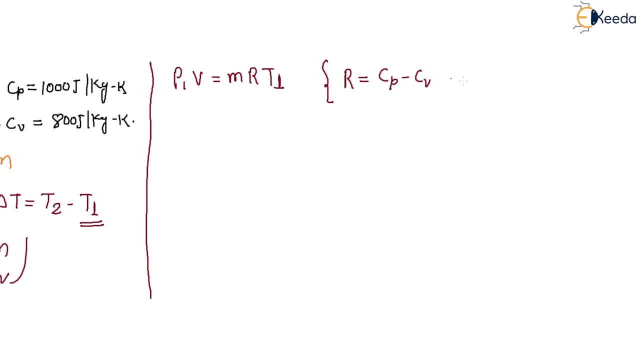 CP minus CV. So you have CP 1000.. You have CV 800.. So what is your 0.2 kilojoule per kg Kelvin? So what is P1?? P1 is what P1 is, given 10 to the 5 Pascal. So what is the kilo Pascal? 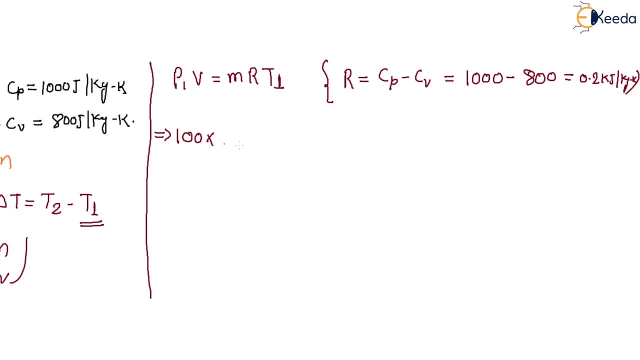 100 kilo Pascal? What is volume 1 meter cube? What is mass 1 kg? What is R 0.2? and it is 51.. So what is its initial temperature? Its initial temperature is 500 Kelvin. 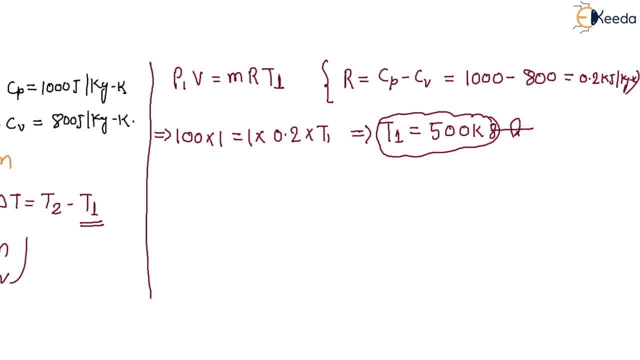 Now, at this temperature you start up the system, So its temperature will increase. So how can you calculate the temperature in the system? Apply first law of thermodynamics. So first law of thermodynamics, Q minus W is equal to delta U, Right? So there is no any heat transfer. So this is 0. Right. So minus of input shaft work is equal to delta U. So delta U is equal to shaft work. 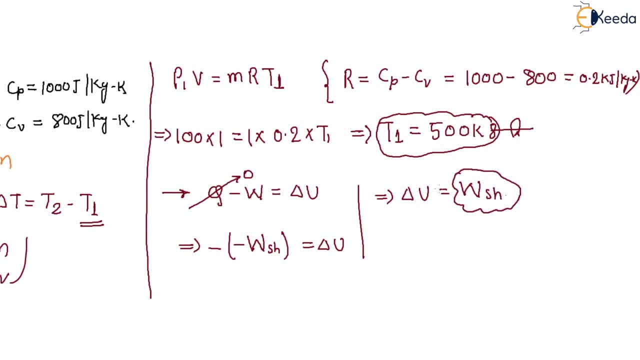 Now, what is the shaft work? Shaft work. If there is a shaft, See if there is a shaft, Apply a torque T Right. Apply a torque T And during application of torque its rotation is 1000 rotation Right. So work done by the shaft on the system is equal to T into theta. 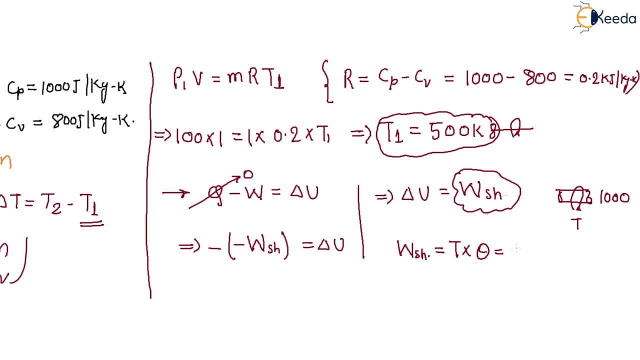 What is the torque? What is the T? 100 Newton meter is the torque. What is the theta? Theta is the rotation. So this is your 2 pi, How much rotation 1000.. So this is your theta, This is your theta Right. So what is your torque? 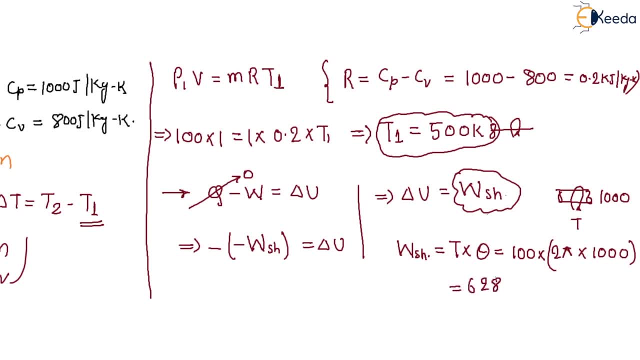 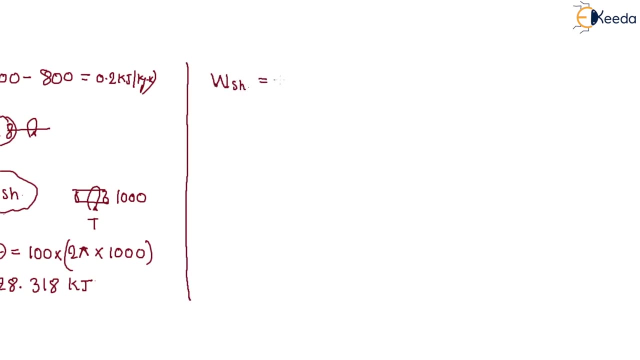 628.3.. 628.318 kilojoules. This is shaft work, which is input to the system. So this shaft work is equal to change in internal energy. That means MCV T2 minus T1.. What is the shaft work? 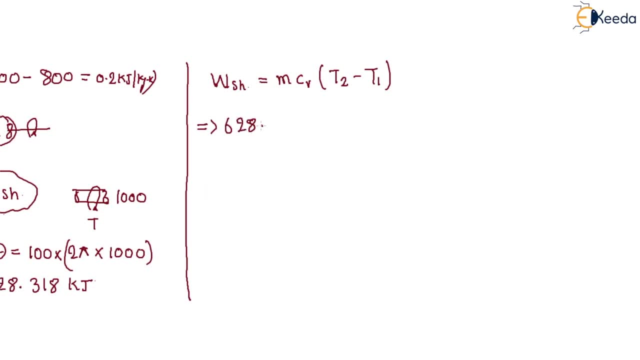 628.318 kilojoules. What is the shaft work: 628.318 kilojoules. What is the mass? 628.318 kilojoules. What is the mass: 1.. What is the CV? 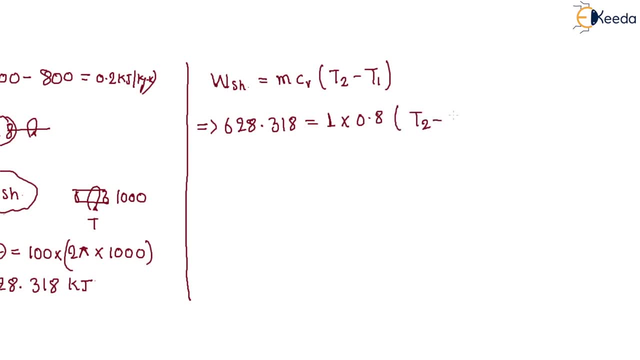 0.8.. What is the temperature T2? I don't know. What is the temperature T1? 500.. So final temperature is what? T2 is what? 128.5 point: See, There is a container.